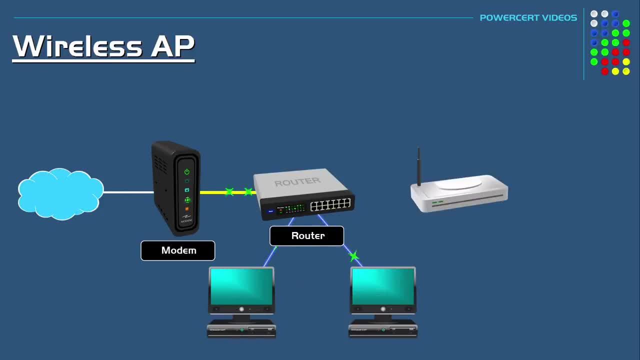 a wireless access point. A wireless AP relays data to the internet and then it connects to the internet. This is the connection between the wireless network and the wireless devices. It's basically a wireless hub that's used by wireless devices to connect to an existing 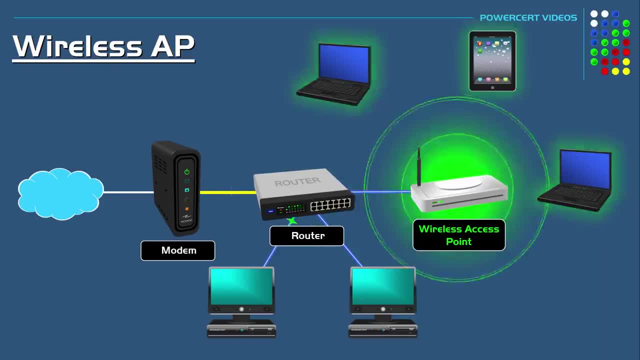 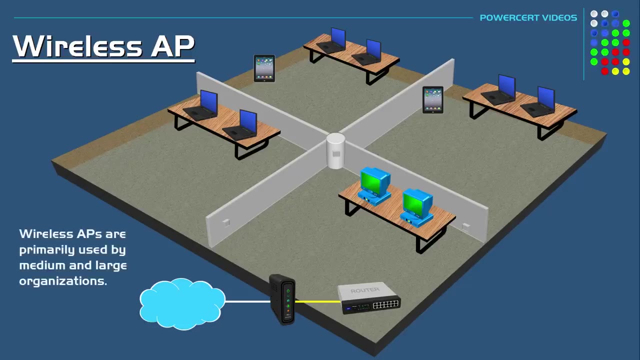 wired network. A wireless AP connects directly to an organization's router, where the router is then connected directly to a modem, which gives the wireless devices access to the internet. Now, wireless access points are primarily used by medium to large organizations and typically an. 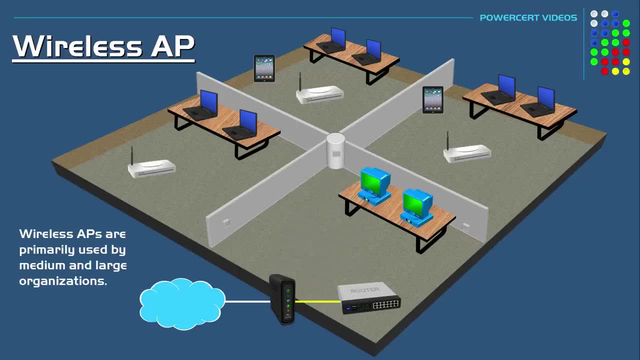 organization will have multiple access points to make sure it covers the entire building. So, for example, here we have a medium-sized office and this office has desktop computers, laptops and tablets. So the desktop computers will connect to the organization's router using ethernet cables, But in order for the wireless laptops and tablets to connect to the network, 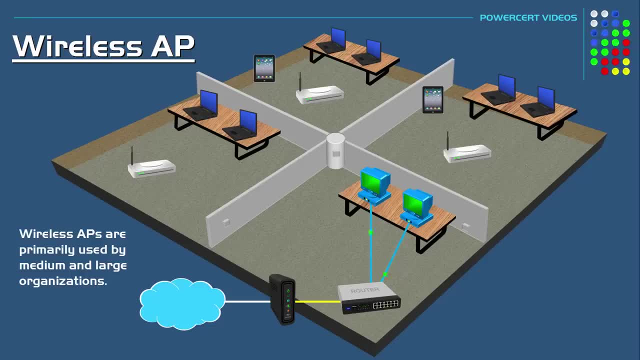 this office is going to use wireless access points, So the access points are going to be placed in strategic places and each of them will connect to the router using an ethernet cable. Then, once that is done, they will all broadcast a wi-fi signal so that the laptops and tablets can connect. 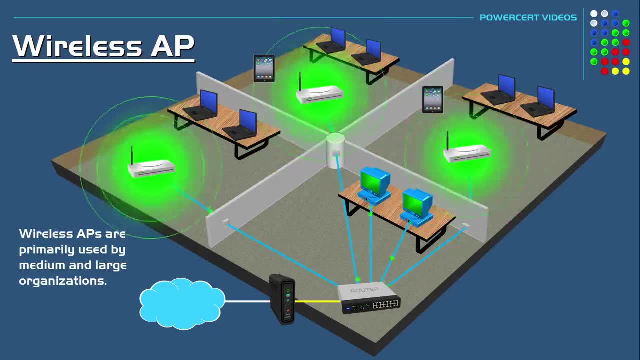 wirelessly and join this network. So now all the desktop computers and wireless devices are joined together in one network and that one network is managed by one single router. And because wireless access points are managed And because wireless access points are managed by a single router, That is one of the main reasons why larger organizations use wireless access. 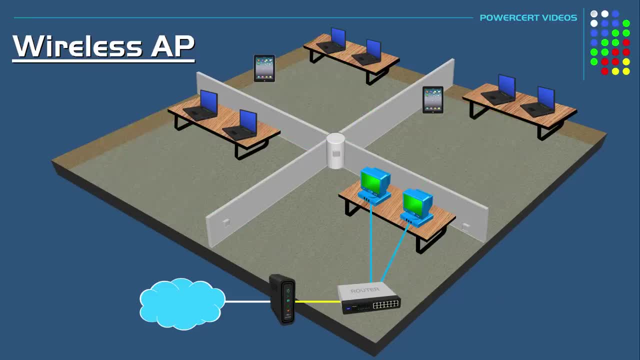 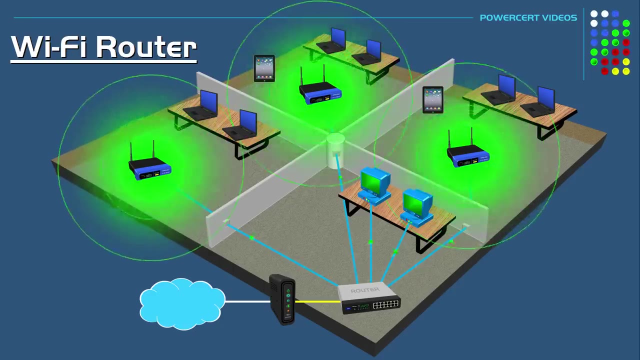 points instead of Wi-Fi routers. Now, in reality, this office here can use Wi-Fi routers instead of wireless APs and it would work just fine. But the problem with using Wi-Fi routers instead of wireless APs is manageability. If the network administrator wanted to manage this network and 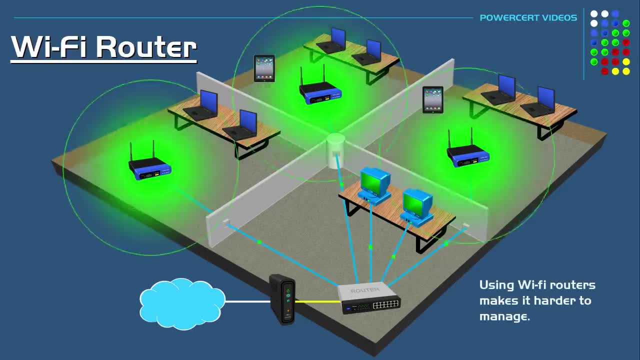 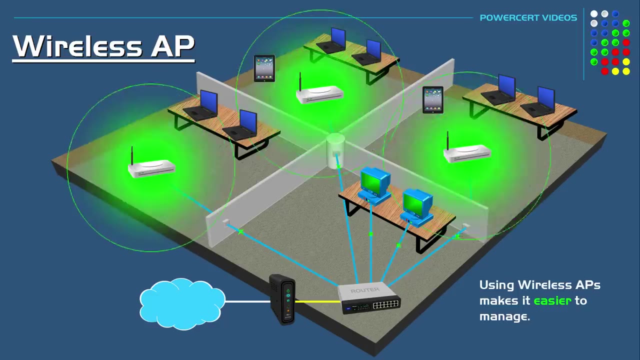 make certain changes, he would have to log into each Wi-Fi router to make that change And that could be a hassle and time consuming, especially if there were a lot of Wi-Fi routers. But if this office was using wireless access points instead, then all the management and all the changes in 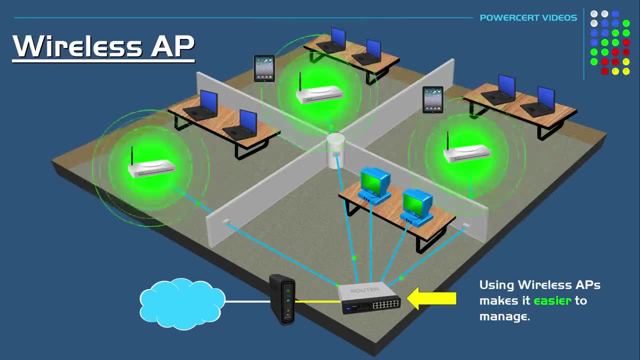 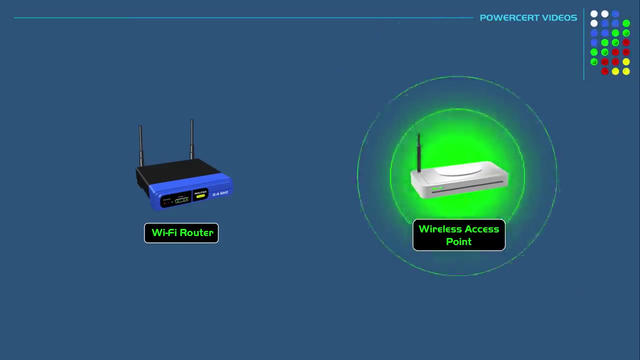 the configuration would be done by this single router, which makes managing a network a lot easier, So all the wireless devices can be treated as a single subnetwork Instead of being treated as multiple subnets if Wi-Fi routers were used. Another difference between these is how devices are able to connect to them. Wireless access points are strictly for. 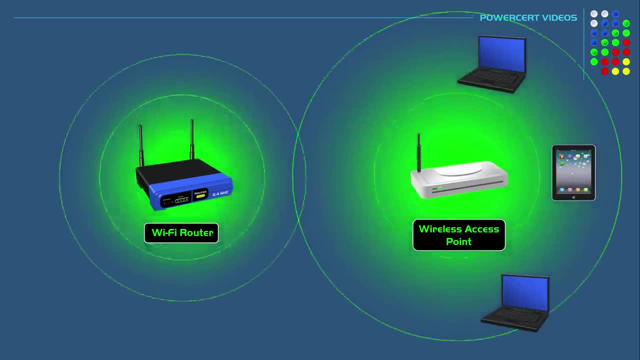 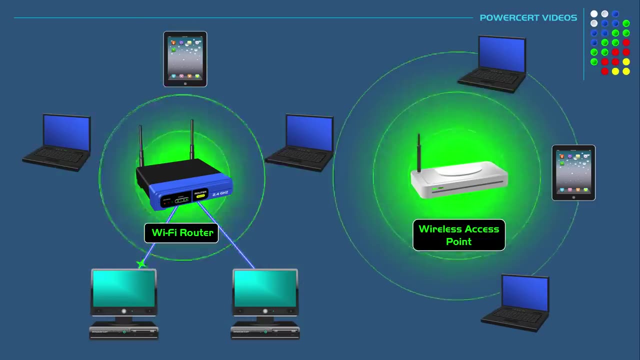 wireless devices to connect to, whereas Wi-Fi routers are able to accept connections from both wireless devices and wired devices Because, in addition to having a Wi-Fi antenna, Wi-Fi routers will also have a built-in switch to accept Ethernet cable connections. Another difference is a firewall. Wireless access points don't have 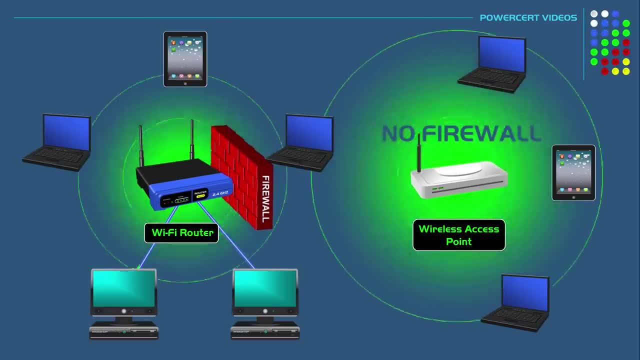 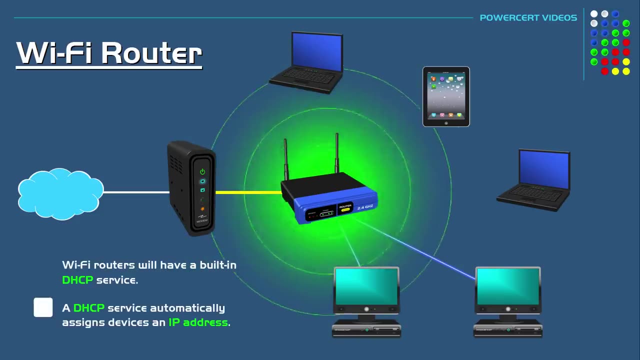 a firewall. while Wi-Fi routers will have a firewall, Wi-Fi routers will also have a built-in DHCP service. A DHCP service is what automatically assigns IP addresses to devices that are connected to it. So when devices connect to a Wi-Fi router, its built-in DHCP service will 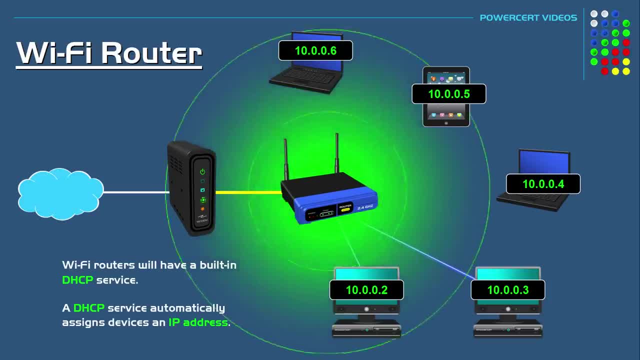 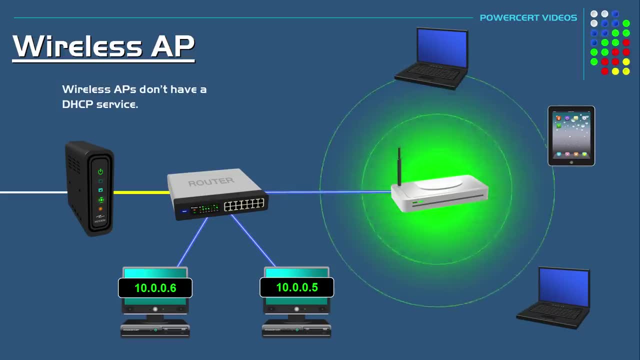 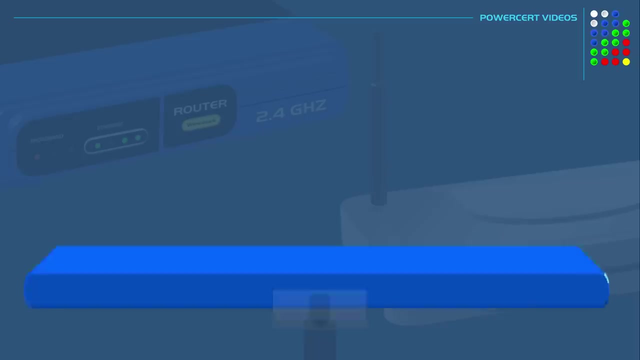 directly assign those devices an IP address. But since wireless APs don't have a DHCP service, the devices that are connected to it will get its IP address from the organization's router. So once a device connects to the wireless AP, the router will send the IP through the wireless access point and then to the device And another. 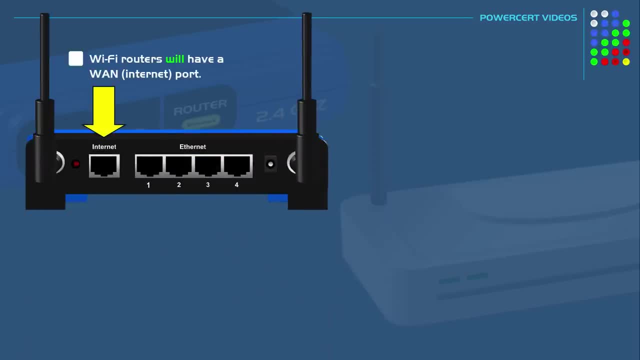 difference is that Wi-Fi routers will have a WAN port or internet port. A WAN or internet port is where you would plug in a network cable coming in from your modem, And this is what gives your Wi-Fi router an internet connection so it can pass it on to other devices, whereas a wireless 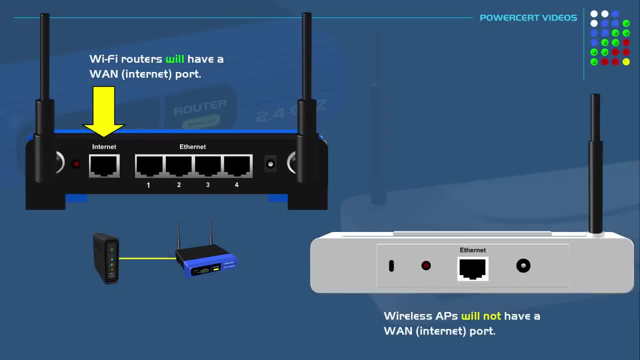 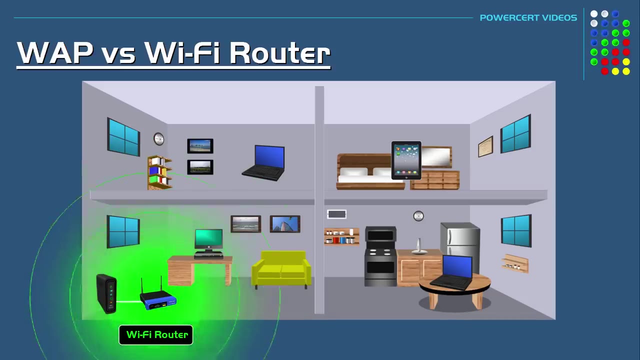 access point doesn't have a WAN or internet port, So it cannot directly connect to a modem. It has to connect directly to a router instead, and then the router is what connects to a modem. And on a final note, wireless access points are often. 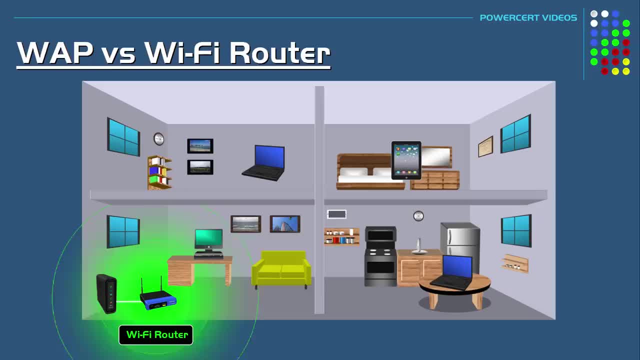 used to connect to the Wi-Fi router. So if you have a Wi-Fi router and you want to connect to a Wi-Fi router, you can connect to the Wi-Fi router using a network cable to the Wi-Fi router. So, for example, if this home needed to extend its Wi-Fi signal further into this home,